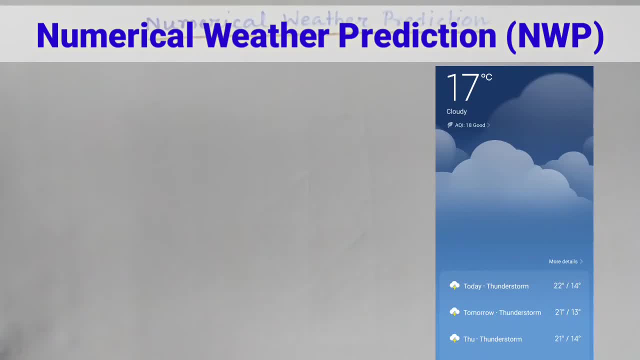 how those can be done. So these type of predictions of weather or forecasting of weather conditions, Weather conditions are done by NWP or numerical weather prediction. This is the most important prediction application of the meteorology. The objective of NWP is to predict the future state of the atmosphere circulations from: 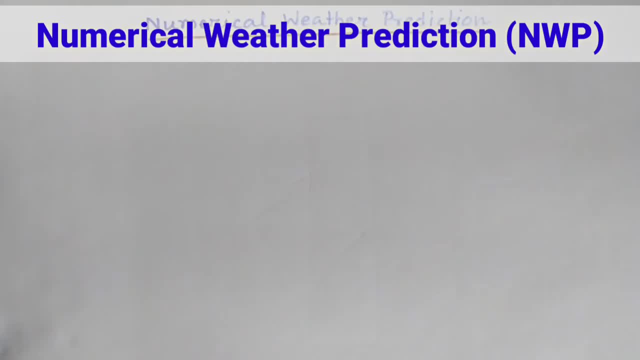 the knowledge of the current atmospheric state by using the dynamical equations. So we will discuss about these dynamical equations later in detail. The three main information required for NWP are: initial state of the field variables. a closed set of prediction equations. a method of integration. the equations in time to obtain. 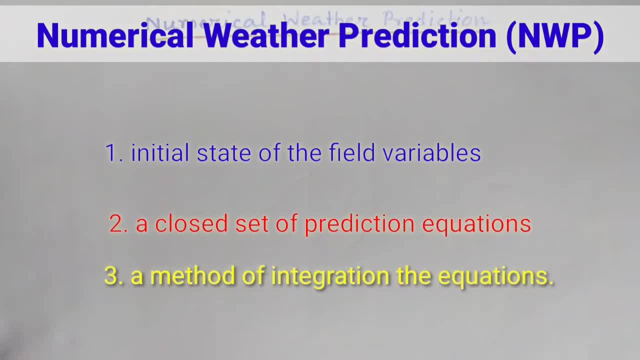 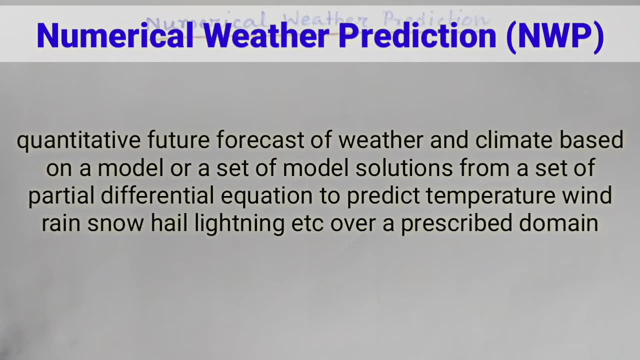 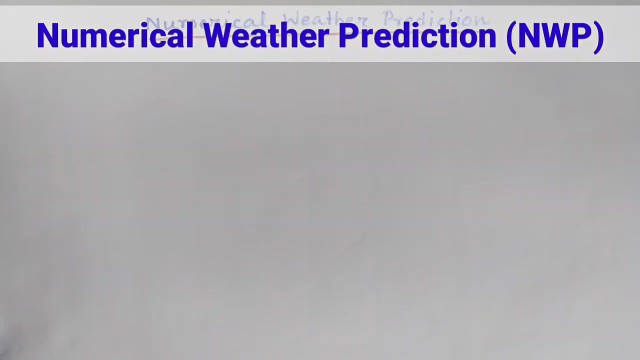 the future field variables. Thus NWP is quantitative future forecast: A set of model solutions from a set of partial differential equations to predict temperature, wind, rain, snow, hail, lightning, etc. over a prescribed domain. Prescribed domain means over a particular region of the earth or maybe the full globe. 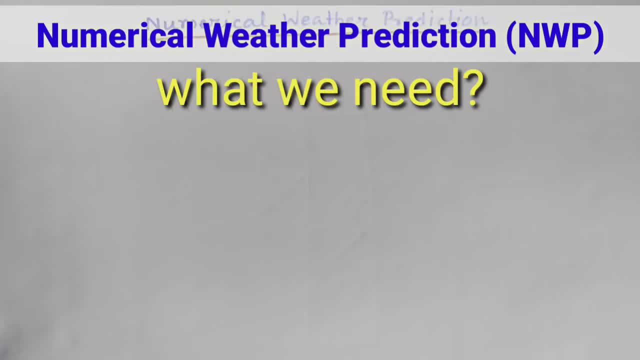 So for that what we need: 1. Partial differential equations, like partial differential equations describing the dynamics of the atmosphere. 2. Numerical approximations. We need to approximate those numerical values because those set of equations cannot give accurate results. So we need to give some approximations. 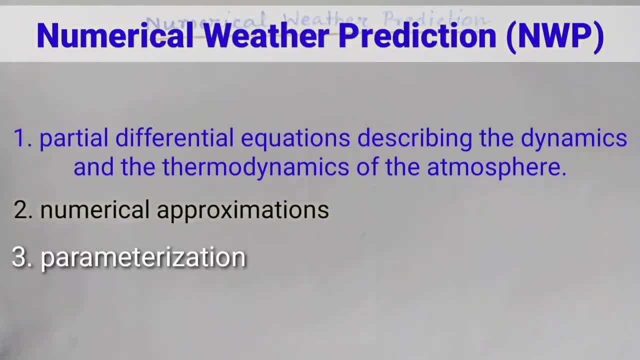 3. After that parameterization, Each and every point I will discuss in detail later- 4. After that, we need a domain, 5. And the domain configuration, 6. And finally, we need initial and boundary conditions. Before going for the details of these components I will introduce, just I'll give some historical. 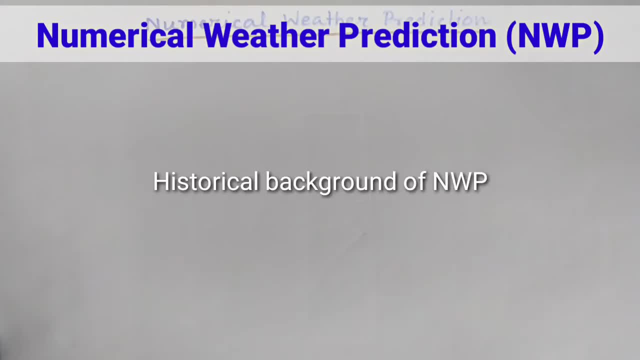 background about this numerical weather prediction, how it is developed from the past history. In 1643, first it was invention was there By Torricelli. barometer was invented. After that, 1850-1902, primary ideas of numerical weather prediction grew during this period. 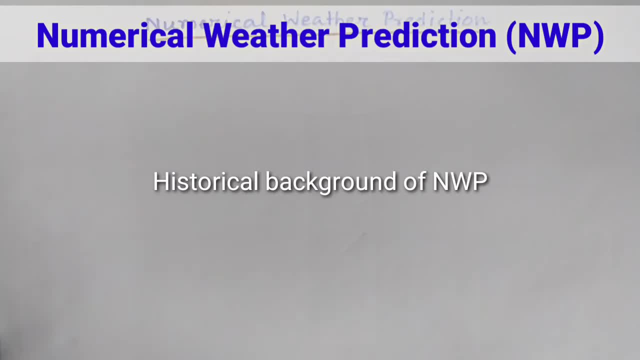 In 1904, we Bajerkens recognized that numerical weather prediction is an initial value problem. Before that, some scientists were trying to solve the problem of initial value. Before that, some scientists were trying to solve the problem of initial value. 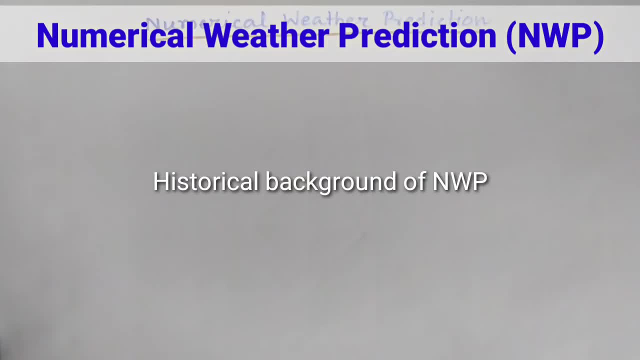 But it was very complicated. But in first Bajerkens recognized that it is a initial value problem. The basic set of equations is very complicated with highly non-linear terms and this partial differential equations do not process closed solutions. That's why there was this idea came by Bajerkens that it it can be solved with the help of. 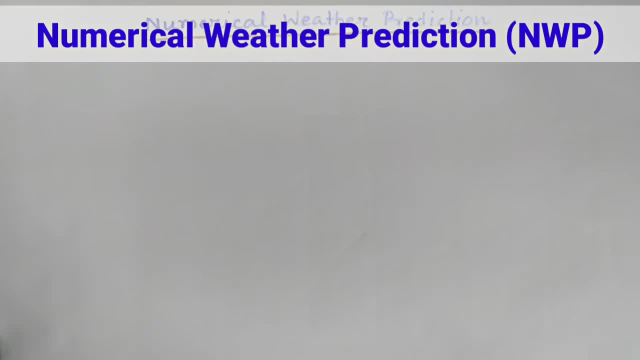 certain variables. that it is. it can be done by initial value problem. However, that time the there was insufficient data about the initial conditions. Later, 1922, LF Richardson solved the system of equations by desk calculator, but it was very complicated. He took around two years to solve the equations. 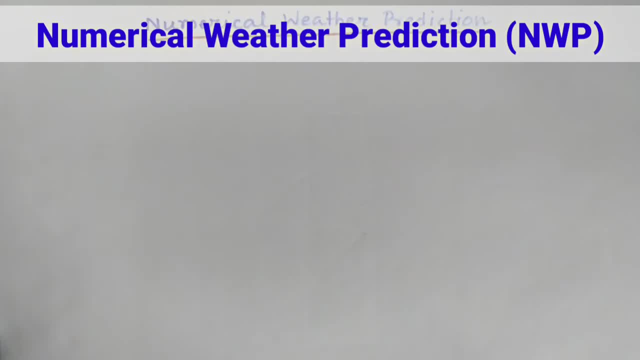 and of course this was a failure, complete failure, but it was giving the basic idea about the next step of the numerical weather prediction In 1930, inventions of radio sundry for upper air data has been invented, so that time it gave a very valuable input about the boundary. 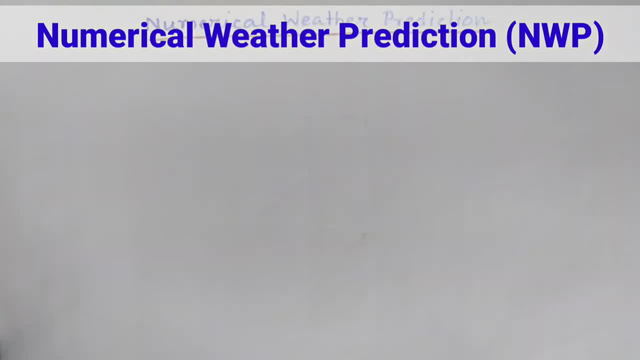 conditions. Nowadays, satellite observations, ground observations, balloon and high performance computers are giving a huge improvements on numerical weather predictions. Now, this was the historical background about this numerical weather prediction. Next step, we will discuss about the equations and how those equations are coming from which? 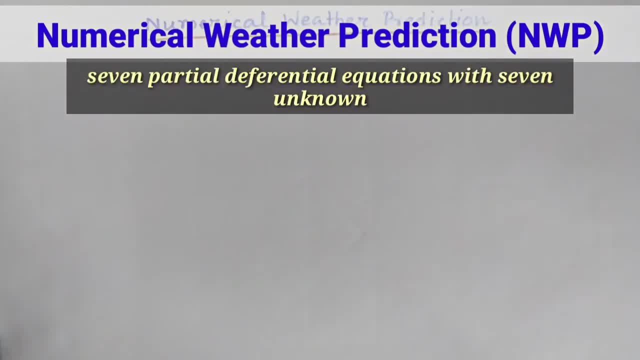 parameters, those we will discuss in detail. There are seven equations. with seven unknowns. We can define theizens that governs the evolution of the atmosphere. that means, with that seven equations with seven unknown variables, we can define most of the dynamical and thermonuclear conditions of the atmosphere. So number one, 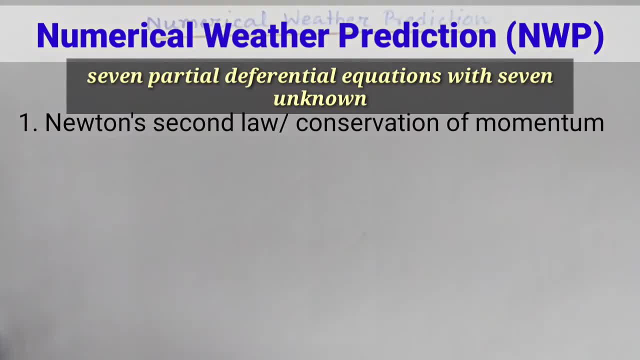 equation is Newton's second law, or conservation of momentum. So first is Newton's second law, or conservation of momentum. Here we get three equations for three component of the entire atmosphere. The first equation is Newton's second law, or continuation of momentum, So salvation of the atmosphere, so thiservation oflines. the relationship, Therefore, the simulation of the 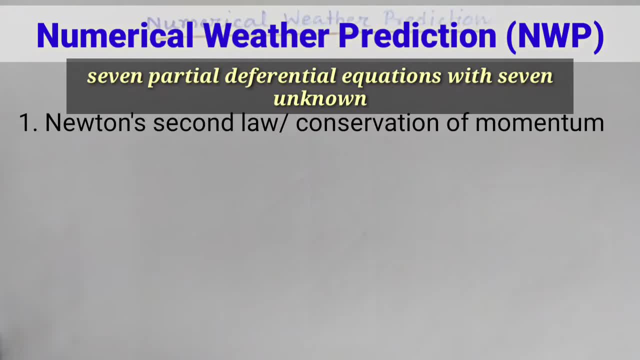 axis, x axis, y axis and z axis. okay, so three velocity component will give three equations for momentum, which gives a newton's second law or conservation of momentum. number two is the continuity equations, or the conservation of mass. number three is the equation of state for ideal gas. already we know the ideal gas equation, that 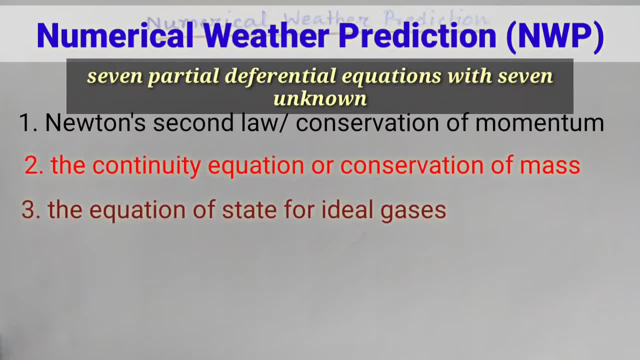 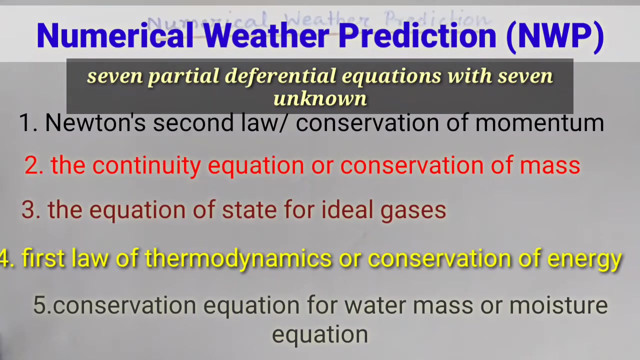 is also will be used in numerical weather prediction. number four is first law of thermodynamics or conservation of energy. so from the first law of thermodynamics we'll use the conservation of energy. that is number four. number five is conservation of equation for water mass. so in the atmosphere initially we are taking the equation of state for ideal gas. there there will 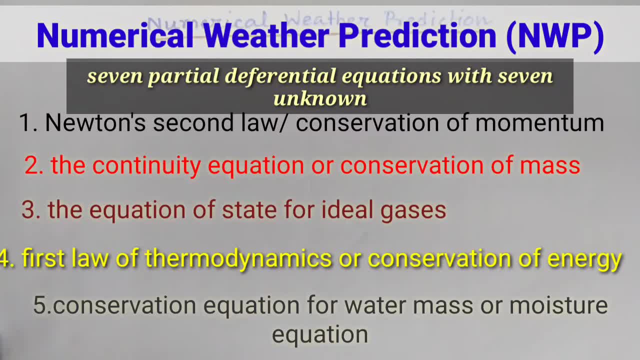 be a dry for the dry air. now, with that, we will use the conservation of energy. that is number four. number five is conservation of energy. that will add the conservation equation for water mass, so as the, in practical case, atmosphere has water vapors and water molecules inside. that's why we need to consider this. 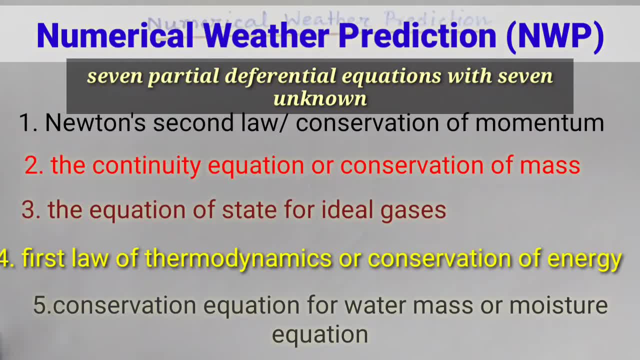 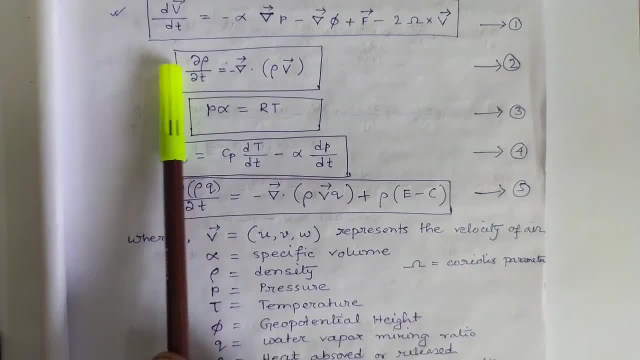 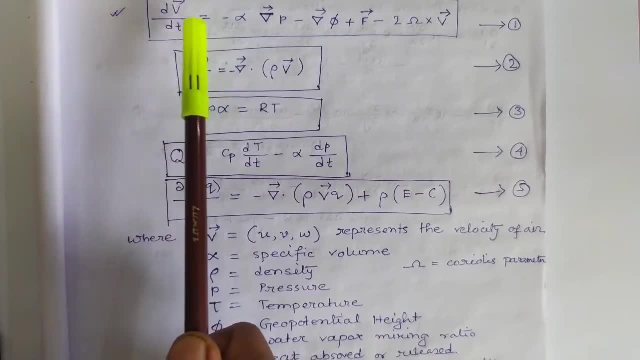 equation, conservation equation for water mass or the moisture equation. sometimes it is also called moisture equation, as i told, the first equation you can see. this is the vector form of the conservation, of conservation of momentum. that is the second law of Newton's second law, dV by dt. rate of change of this velocity, its component with a minus alpha. 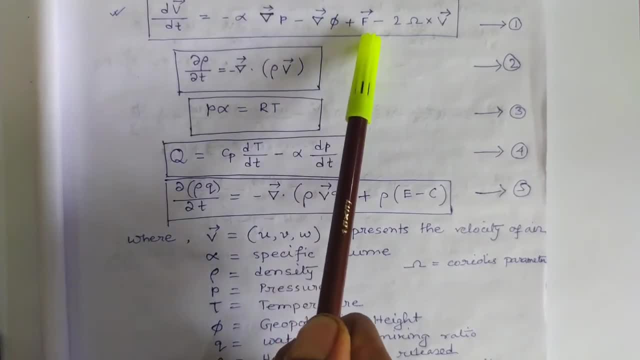 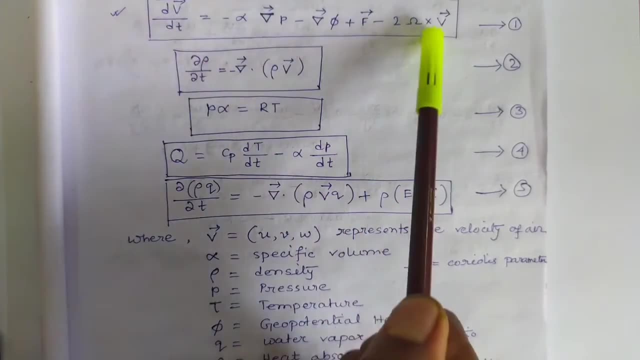 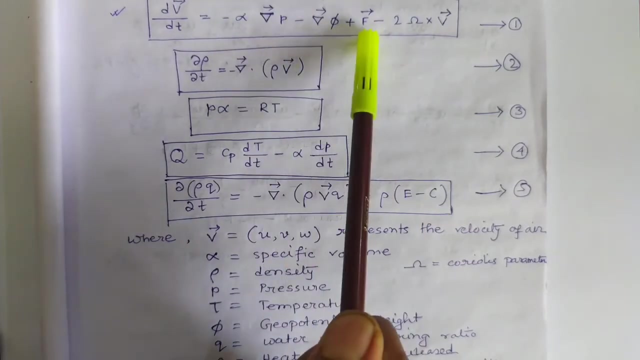 great p minus grad phi plus f minus 2 omega cross v will derive this equation. i think you have already derived in the chapter 1, but still i'll show how this equation came. so which are the every component of the equation? next is the continuity equations. it comes from the fluid dynamics, okay, the density of the rate of change. 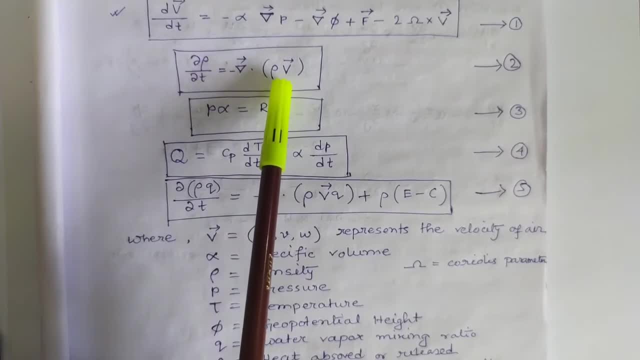 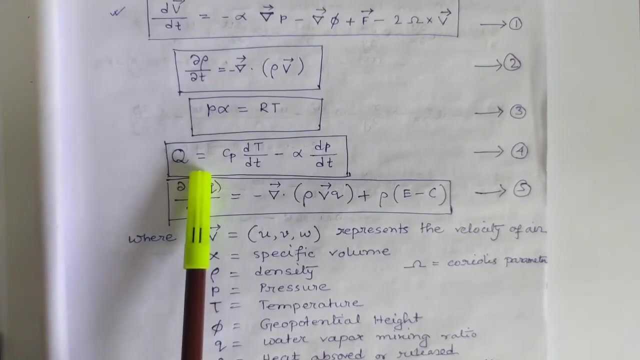 of the density of the fluid is equals to the minus gradient of the rho and rho v. that is the velocity. next we are coming for the real gas, ideal gas equations: p alpha equals to rt, alpha is the specific volume. next we are coming from the thermodynamics: the total change absorbed, or 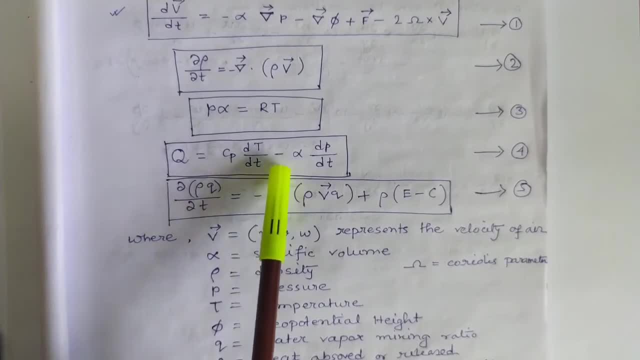 released heat is equals to cp dt by dt minus alpha db dt, that is the rate of change of temperature with time minus alpha rate of change of pressure with time. now the last equation is the moisture equation. it is already you have learned in the micro physical part in the 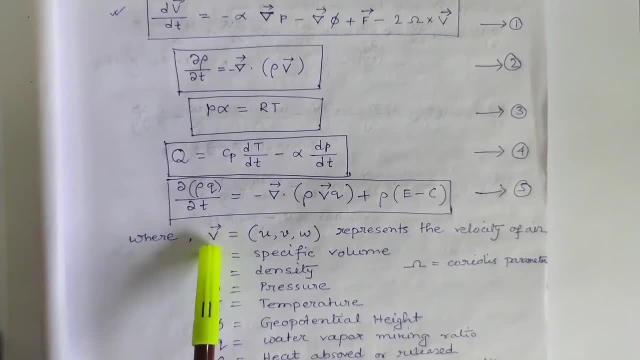 thermodynamics. so here all the convey conventions are used in the. this is the velocity, with three components of velocity: u, v and w, horizontal along the eastward direction, u, v along the north positive northward direction and w is the positive upward direction. now, alpha is the specific volume, rho is the density of the air. here omega is the corollary. 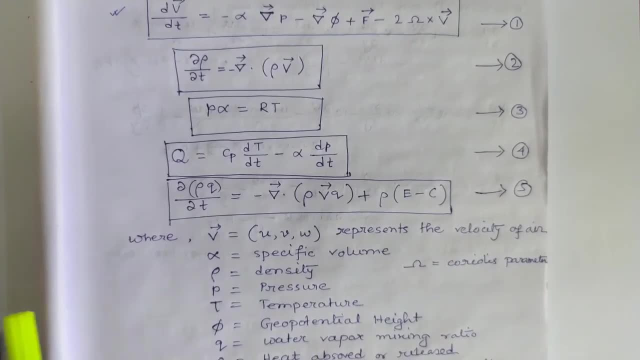 parameter. p is the pressure, t temperature. phi is the potential height, q is the water vapor mixing ratio, now amount of water vapor per unit, volume of unit mass of the air, q is the heat absorbed of the release, e is evaporation. in the last equation we have used evaporation. c is the condensation, r is the real gas constant and 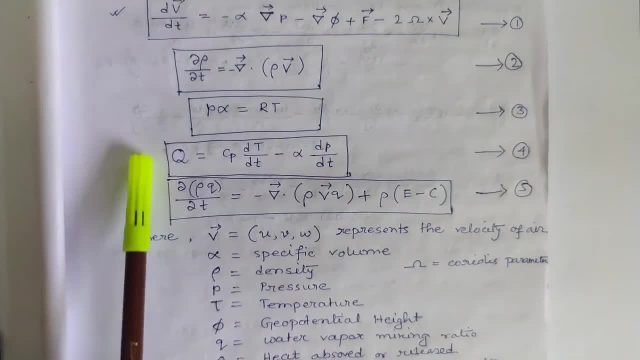 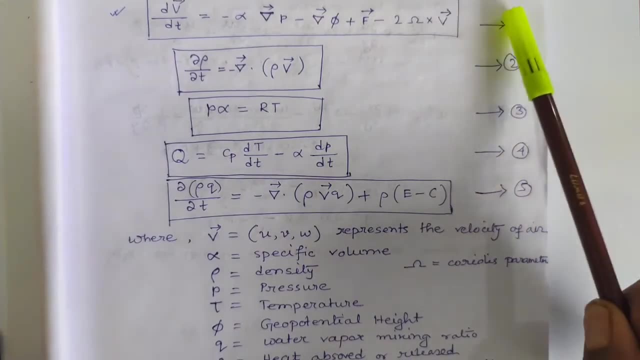 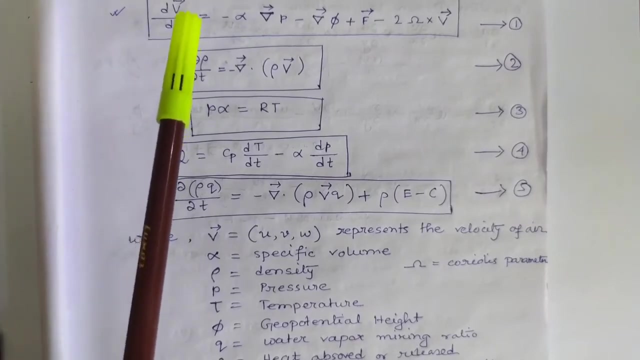 f is the frictional force. so with this here you can see equation one it is. if we describe in different components x, y and z component, then it will be three components of the equation. so three, four, five, six, seven. these seven equations is needed to in the numerical weather. 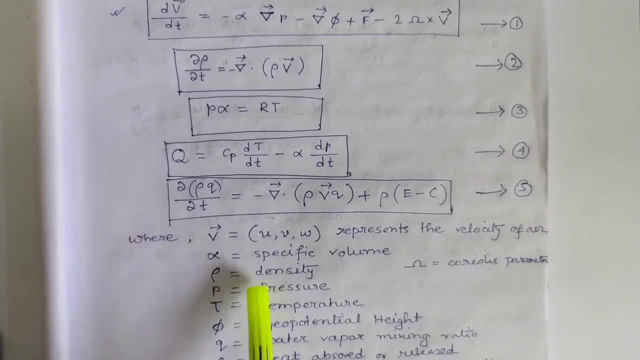 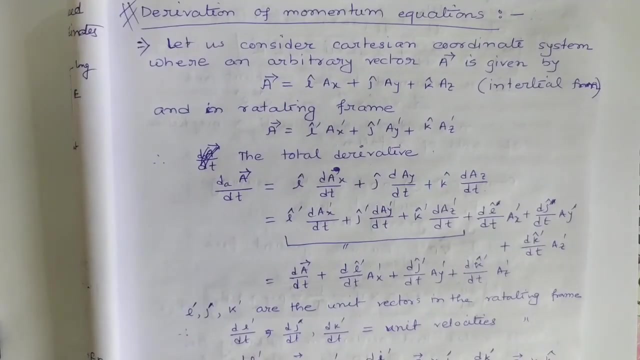 prediction. so for, before going for other parts of the numerical weather predictions, let us see how these equations are coming. so first we'll consider about the equation, equation one. so i'll start from a detailed description. first i'll consider about the rotating frame of reference, because earth is rotating in its axis. so for that we have to make 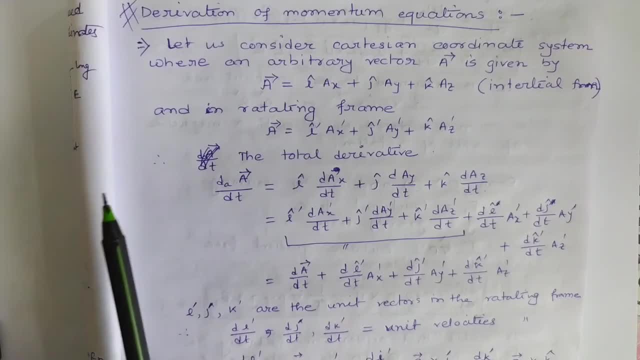 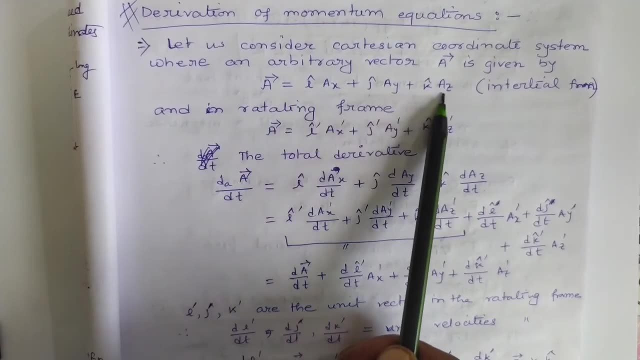 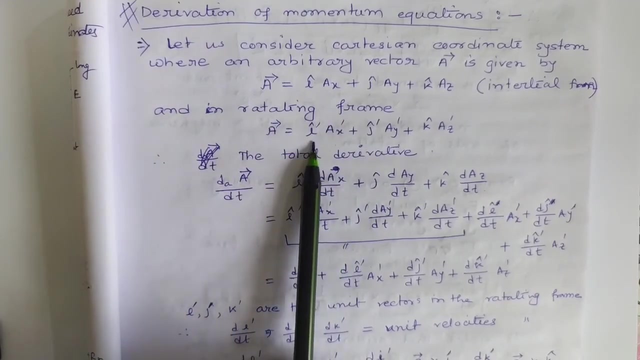 we have to make a relationship between the inertial frame and the rotating frame of reference. so for that let us consider a vector. a is given by this equation that is well known. after that, this a, if it is in rotating frame, then we are representing by i dash, a x dash plus j dash. these are the unit vectors along x, y and z. 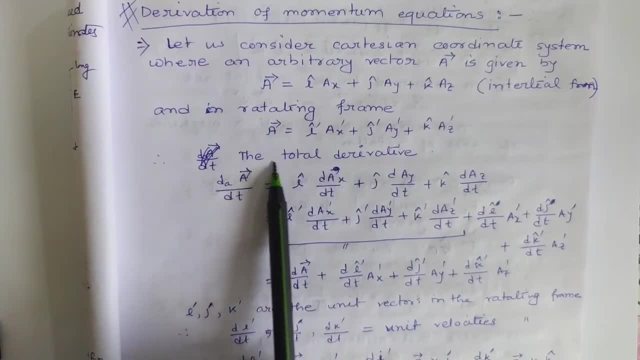 z directions. now the total derivative when we are considering from the opps means rotating frame. the total derivative of a is given by, because i and a, both are changing. i fixed d a, x, d t, j fixed d a, y d t and k fixed d, a, z d t. similarly, 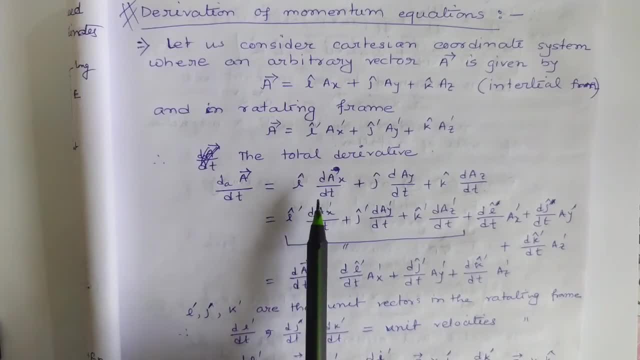 this part again. this can be represented in the rotating frame: i prime, a x prime and similarly other parts here you see i also changing the, i also unit vectors and it is changing. so when a prime is fixed, i is changing, a y prime is fixed, j is changing and a z prime is fixed and k is. 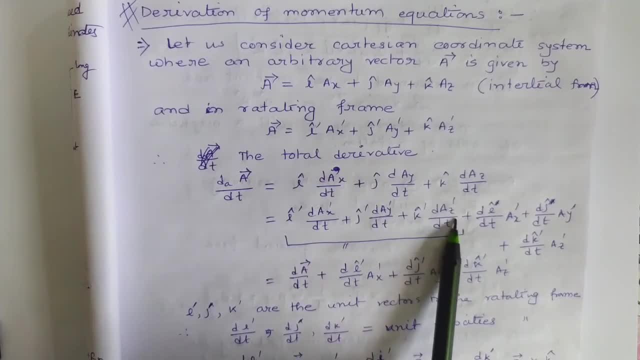 changing with time. now this part you can see this part is similar as d, a, d, t. okay, the left part is this one. now, as i, j and k are the unit vectors in the rotating frame. now, as i, j and k are the unit vectors in the rotating frame. 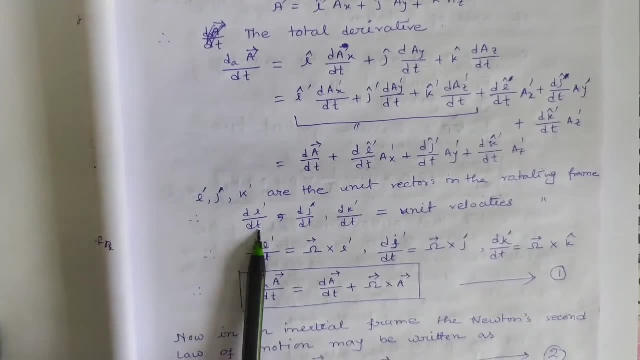 d i dt, d i prime dt, d j prime dt and d k prime dt are the unit velocities along the respective directions. now, so if it is like this, d i prime dt is equals to omega cross i. omega is the angular velocity, so allow similarly j and k. so what we get combining these two equations, d a whole. 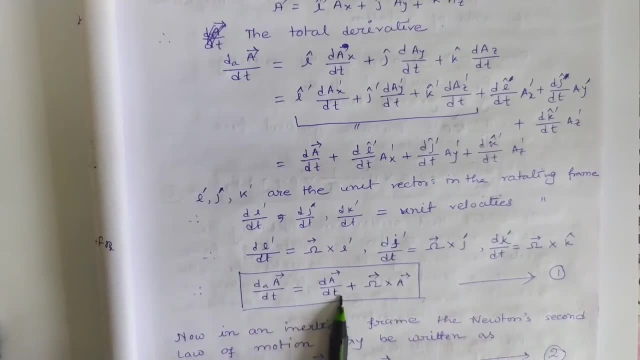 total derivative is equals to the initial frame derivative. this part and this part comes omega, cross a. okay, so i, j and k making the a vector. so this is well known. though it is well known, i am just showing because it will be. this equation will be needing in our 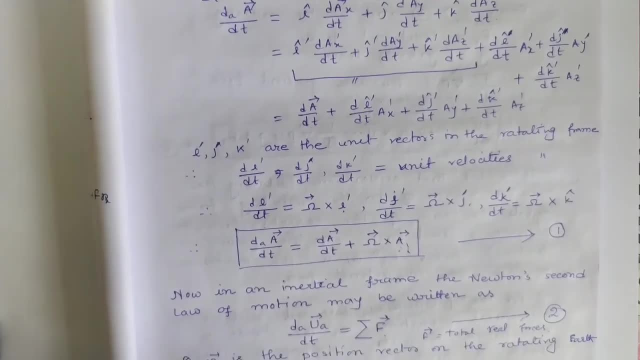 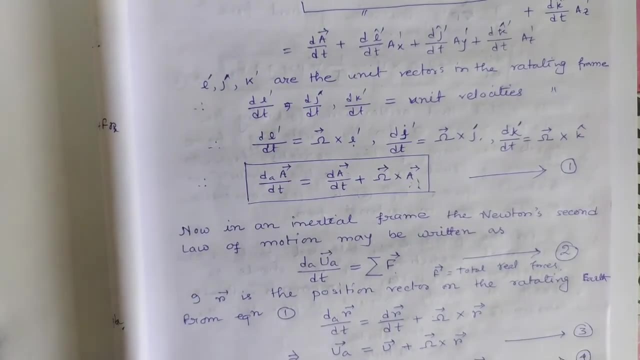 momentum equation. now, second part, we are coming to the. we have to derive the momentum equation. so first we are considering the newton's second law of motion. so newton's second law of motion, in the total derivative, if u, a is the velocity, then we we can write like this: summation of f: so rate of change of momentum is equals to the force, that is. 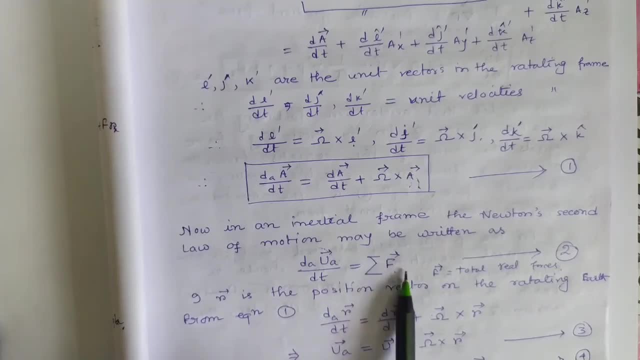 the second law of newton's second law. now this is the total real forces available in the on the earth surface. so this force may come from the different parts, like frictional force, coriolis force. different different parts will come. i will discuss it later now. if r is the position vector on the rotating earth, from rotating earth, that is, from the center. 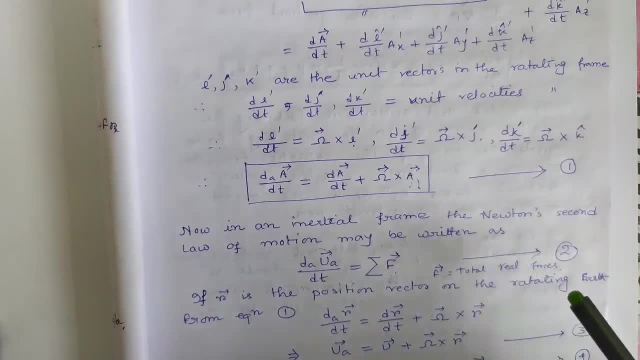 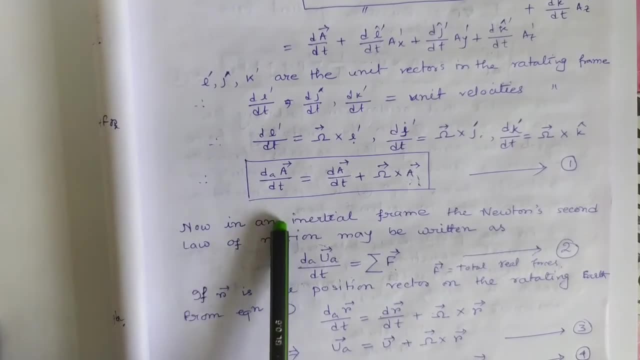 of the earth to the surface at a height. some height it will be there. so we are considering this is a position vector. now, with respect to r, if we use this equation, if we replace by a as any arbitrary vector, so we can put r instead of a. so we are getting like this now: d a. 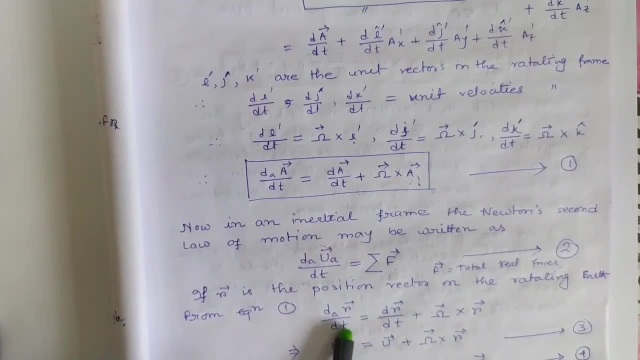 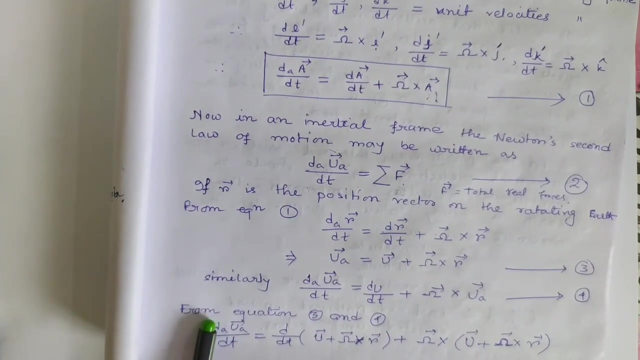 this is the total, this is the velocity component, dr, dt- rate of change of position. similarly we can write this: so in another case, a case, total derivative, we can write like this: so you can see, with this two equation, if we replace we, we put this value here. we are getting okay. so from this two equations you can, we can put the value of u, a here. 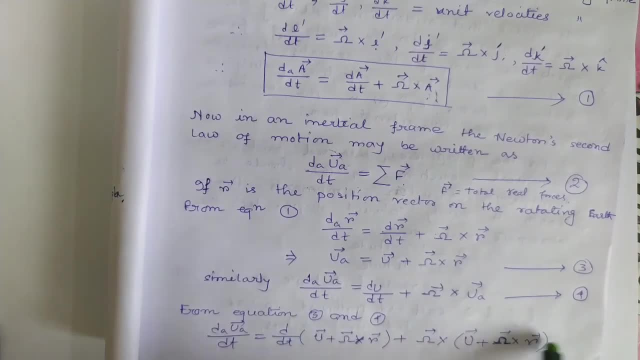 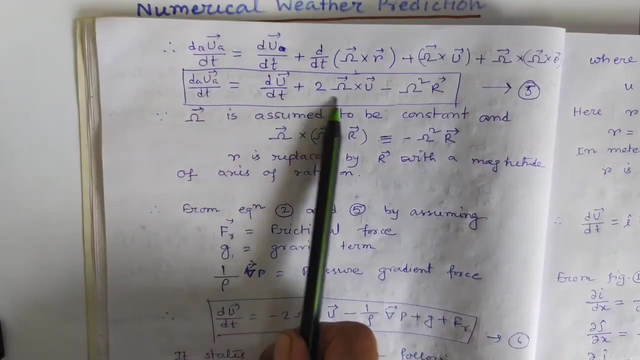 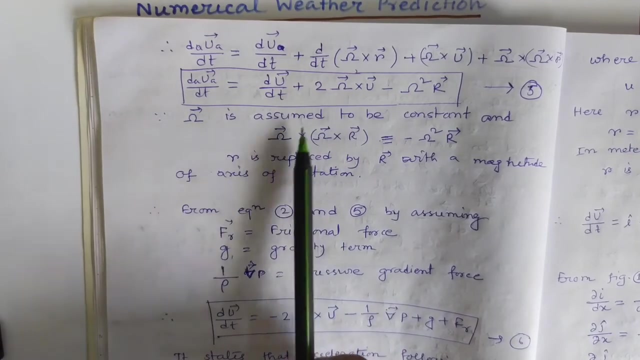 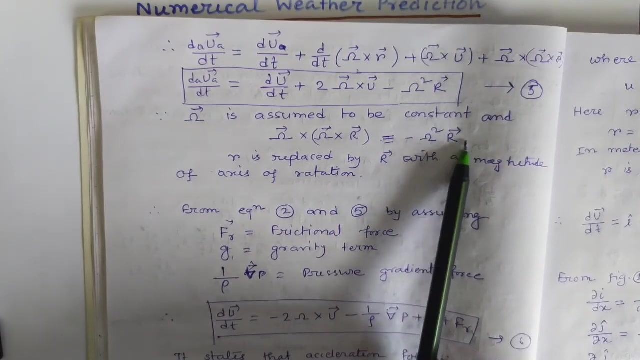 okay, so after putting this value, if you simplify it, we'll get this equation, because here omega is constant and the derivative of omega will be zero, and the other part, omega cross. omega cross r equals to minus omega square r, where capital r we are replacing from the small r. that is the 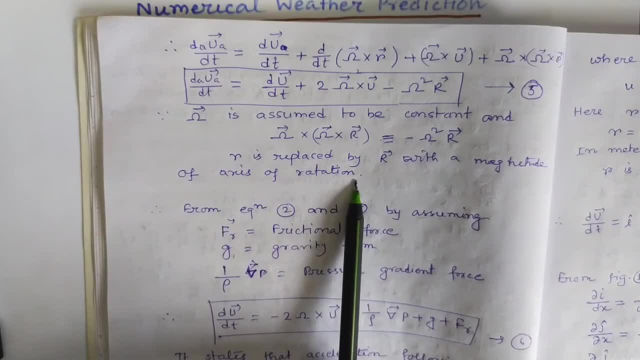 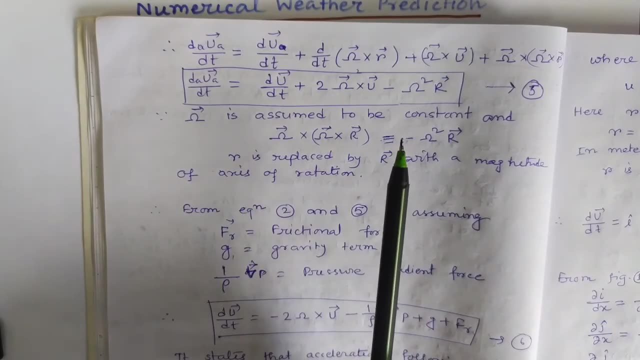 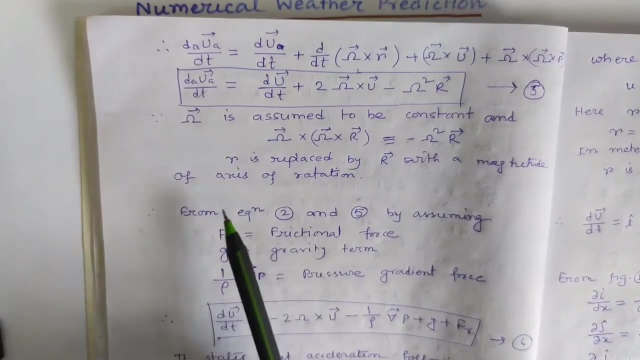 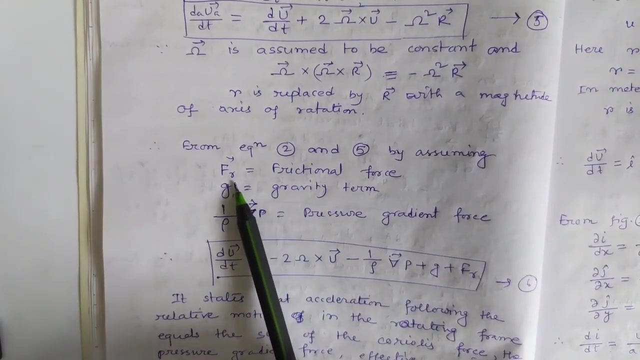 axis of rotation. so r is replaced by capital r with a magnitude of axis of rotation, so as we can replace by any vector, because we are considering the reference frame equation. so now you can see if we consider a frictional force, f, r and g is the gravity term and one by rho, grad, p is the. 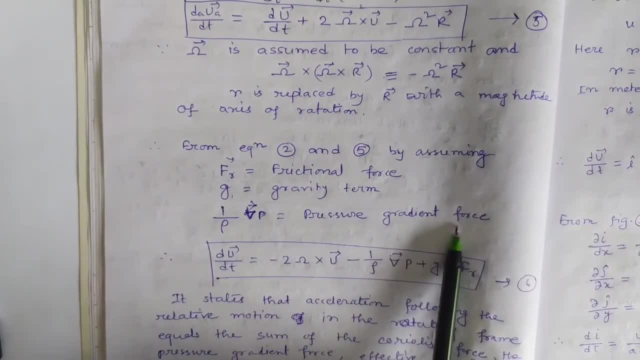 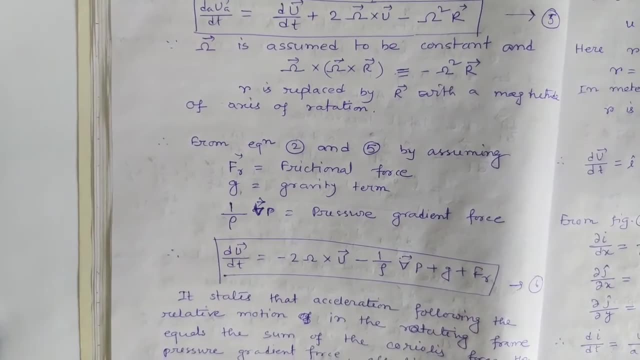 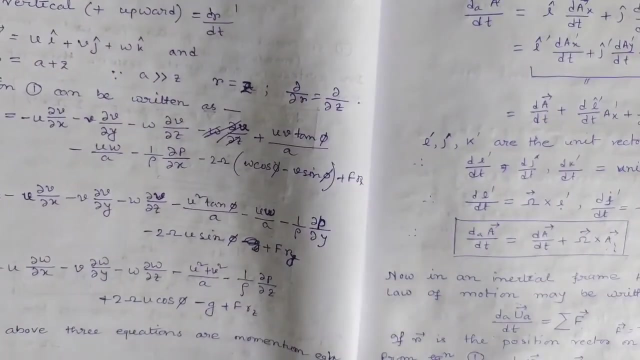 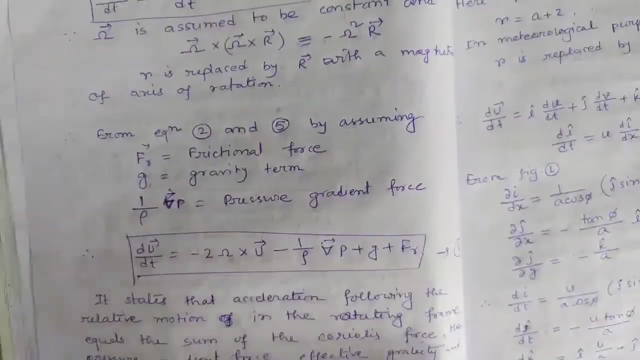 pressure gradient force already you know that is the pressure gradient force. now these components if we put together we will get from equation five and two. so equation two was this equation. you can see this is the equation. so sum of all the forces. so we are considering frictional force, gravitational force and the pressure gradient. 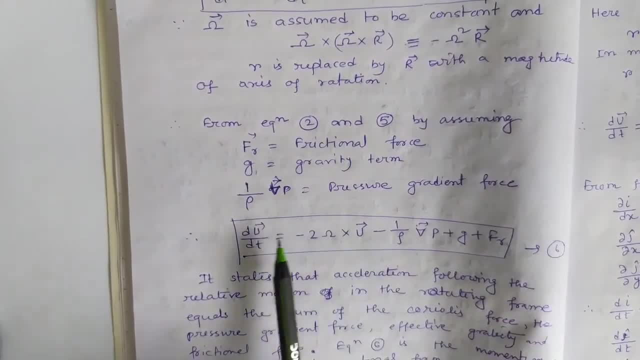 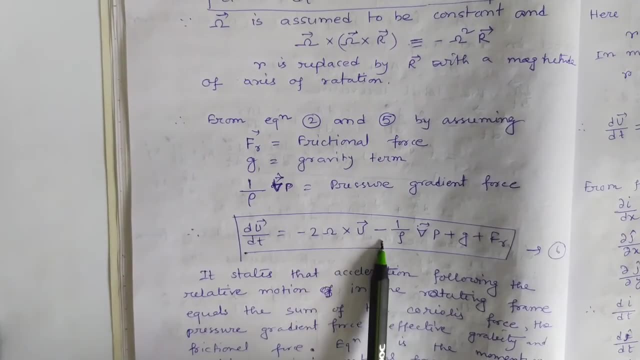 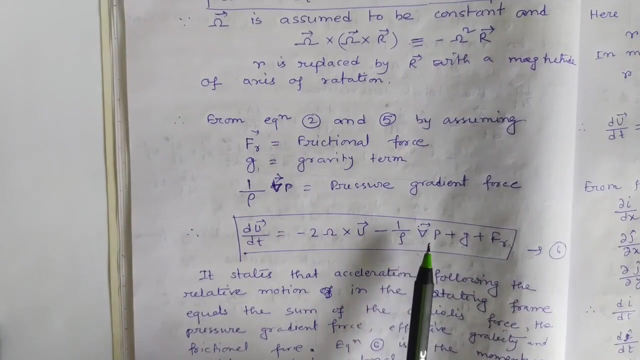 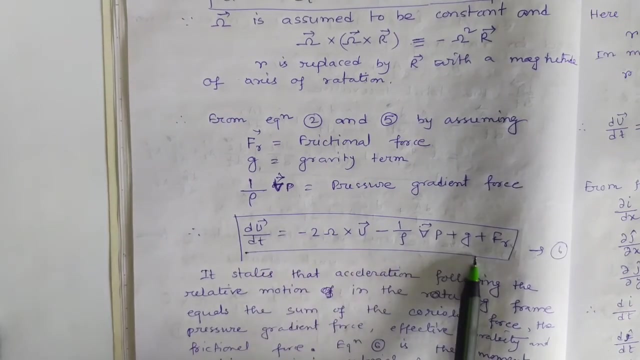 force together. so all the components we are writing here, du dt equals to first term minus two omega cross u minus one by rho grad p plus g plus f r. so all the components like frictional force, gravitational force, pressure, gradient force are assumed here in this equation. okay, 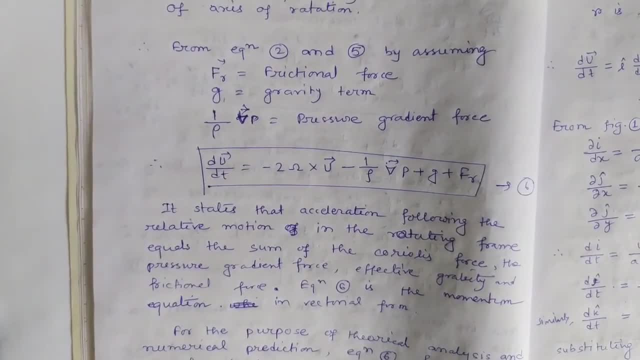 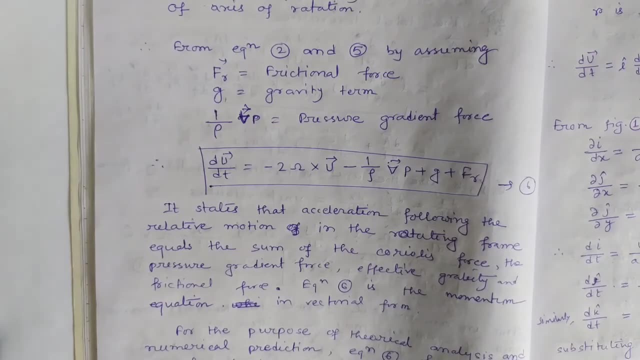 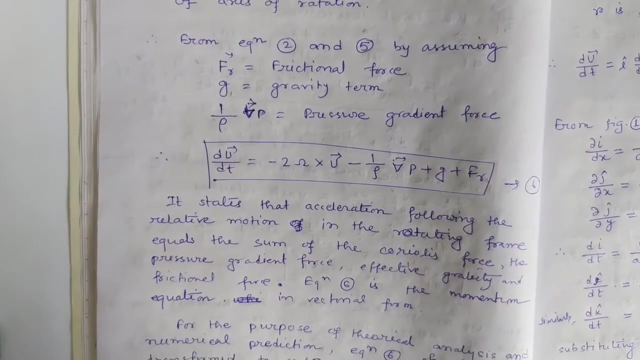 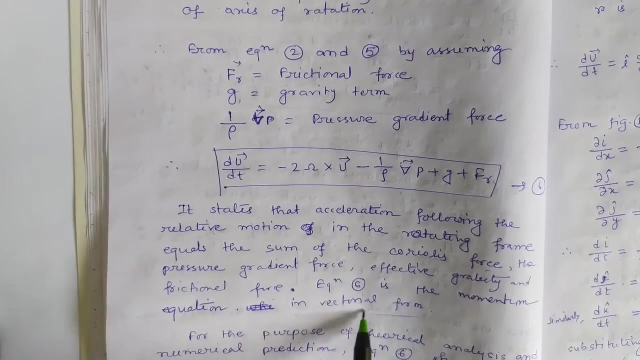 now what it state: that acceleration following the relative motion in the rotating frame equals to the sum of the corollary force, the pressure gradient force and the effective gravity and and frictional force. now this equation is the moment of regression in uh, vectorial form. okay, what we have seen in the 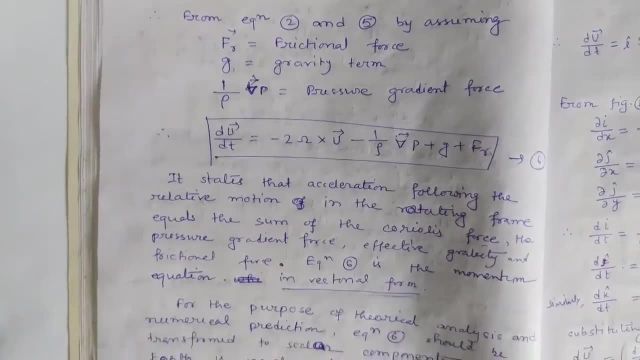 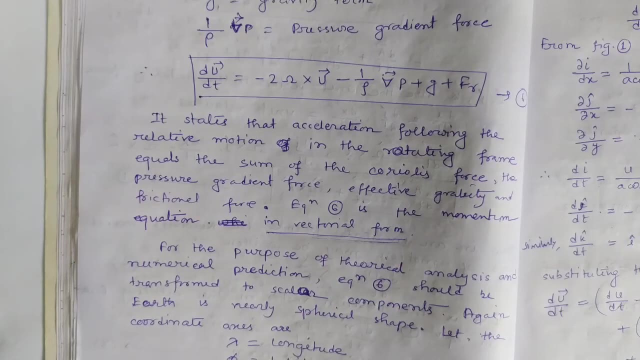 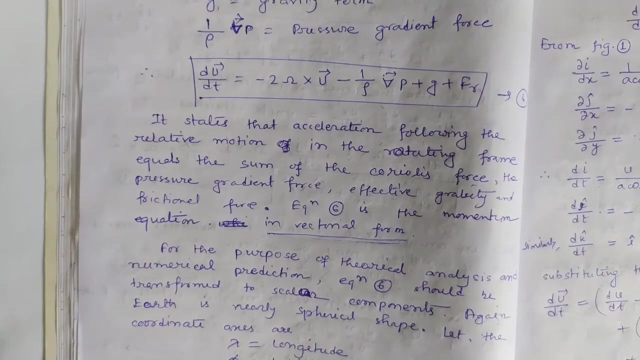 first equation of the nwb. okay, now another thing is in vectorial form, equation cannot be solved practically, it is very difficult. so the components we have to consider, x, y and z components we have to consider, and earth's surface is a earth is a spherical coordinate system. that's why we have to convert this cartesian coordinate system to 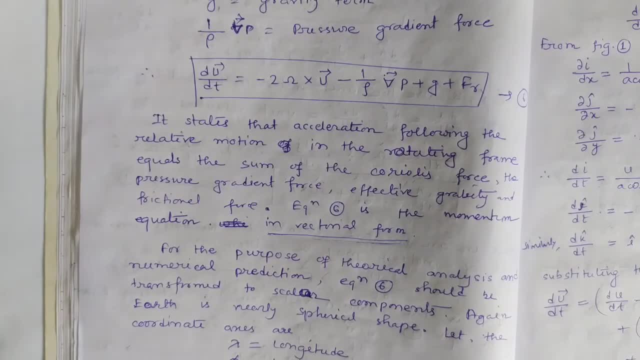 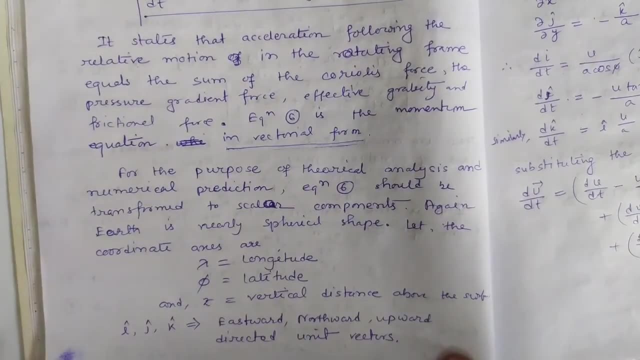 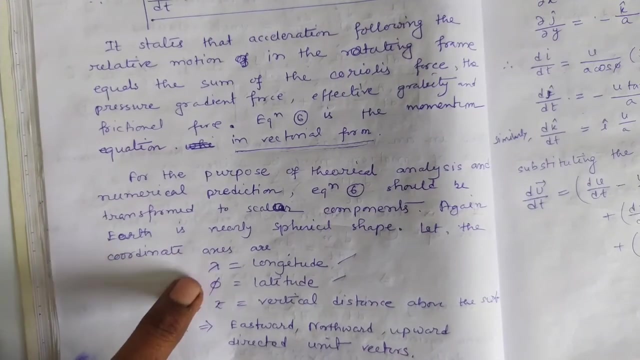 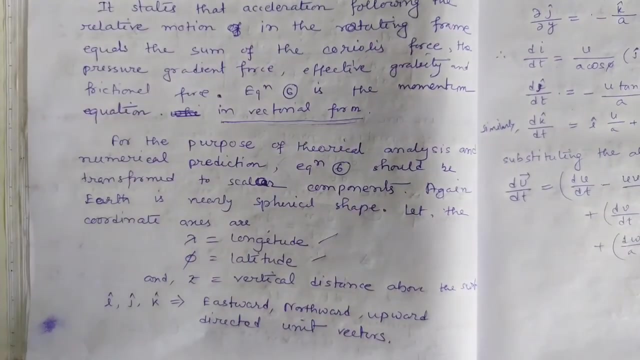 spherical coordinate system first. so for that, let us consider for spherical coordinate system, three components, three axes. we need one is your latitude, longitude and vertical distance. okay, so these are the angle. like in spherical square system, spherical coordinate system, we use theta and phi, here also lambda and phi we are using. z is the vertical distance above the surface. 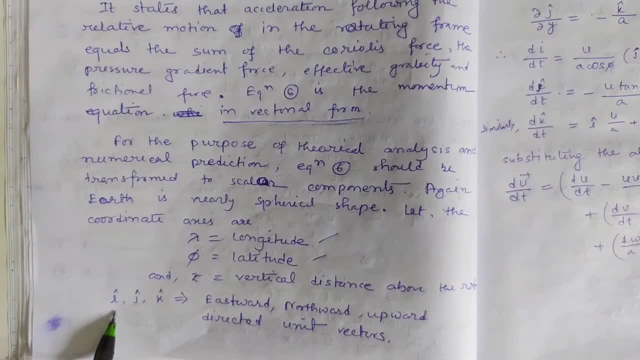 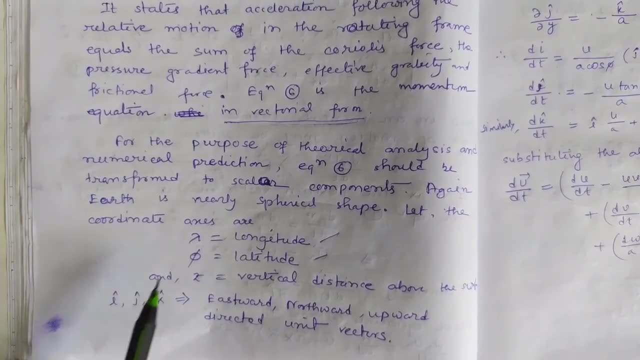 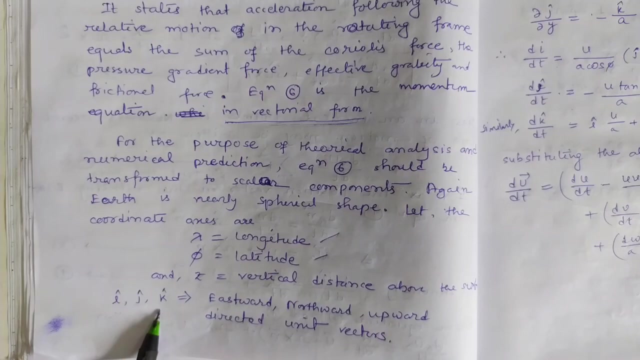 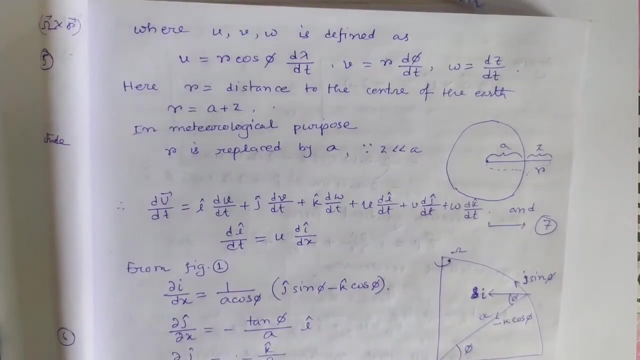 now in unit vectors also changing unit vectors. we are considering eastward, northward, and i 'm going to add pha here for the first variable only pha is faint. that is when the w versus v simple point is f and a, and this is going to be the phase where we have, for short period, 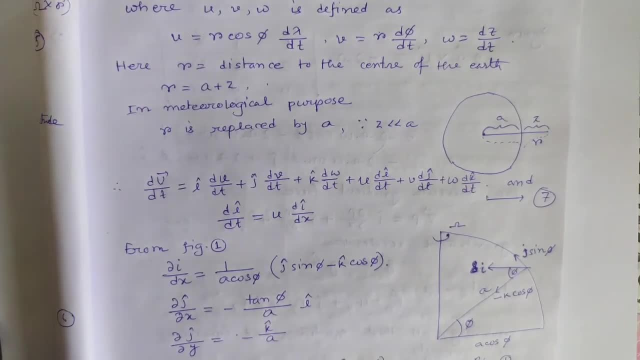 and therefore this will have to beWhi always is basic to actually start with what is light and us. if we find that unit pic Shooting Cloud Bay is m where unusual hit, you will find that in ellipse we have theta. r equals theta, this vertical distance from medium. 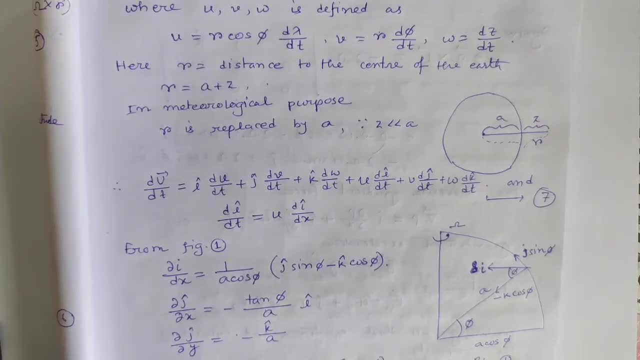 dachte one is h here to theta, here or theta, our r equals to w. so if we define location in antifree pin of the wing, atр is the vehicle weight of weight and negative v is equal to r, d, phi, dt and w is equal to dz, dt. Now, here, distance to the center means r is the. 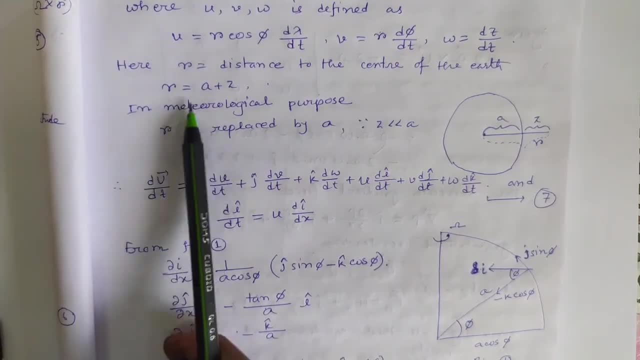 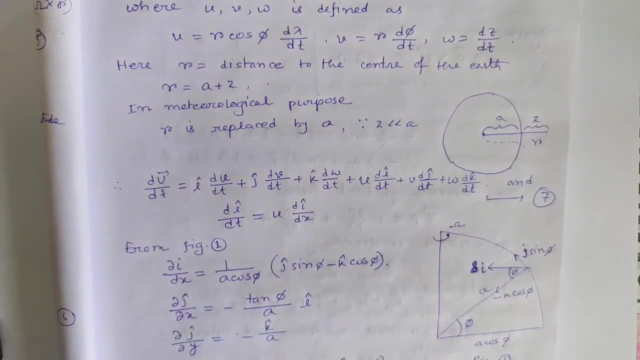 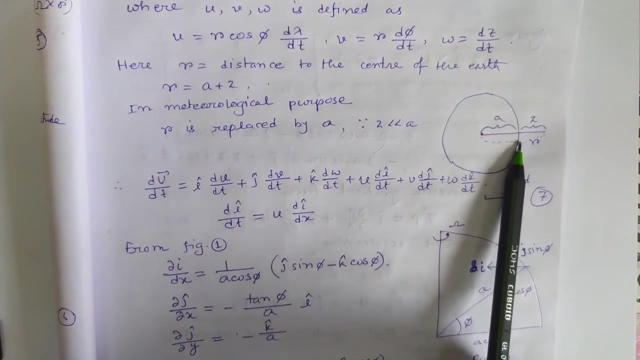 distance to the center of the earth. r is given by a plus z, So a is center to the surface and z is the height from the surface. Now, for meteorological purpose we need very smaller height, So we can replace r by a. okay, We are. we are neglecting z, because z is very small for meteorological purpose. 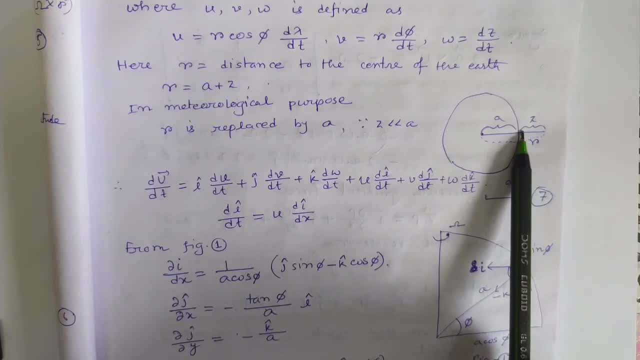 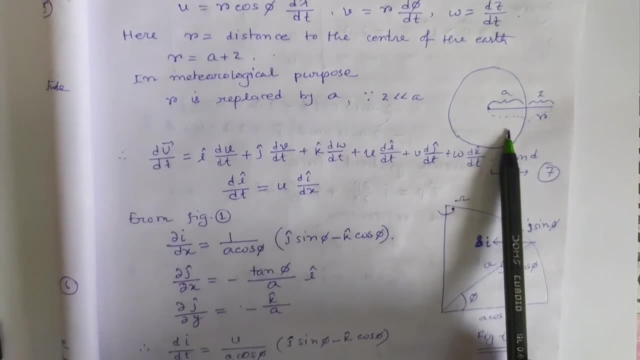 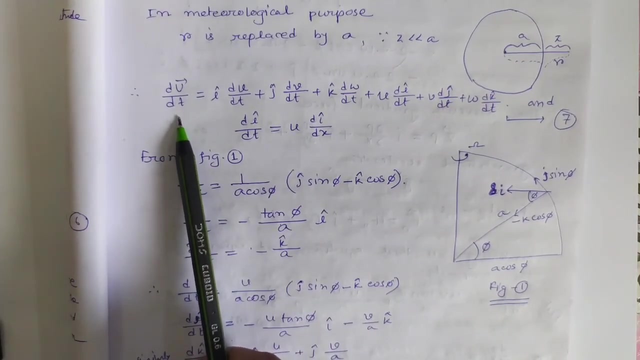 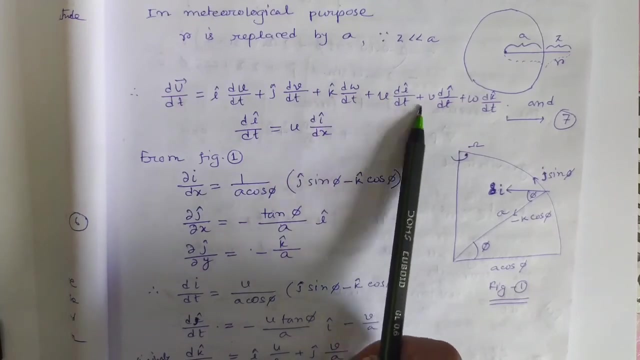 it is very small because we are considering other few, around 20 kilometers, with respect to millions of kilometers here. okay, Now this velocity component, rate of change of velocity can be given by i, d, d, t, z, j, dv, dt, k, dw, dt plus u, di, dt plus v, i, d, dj, dt, w, dk, dt. Here these components, of course. 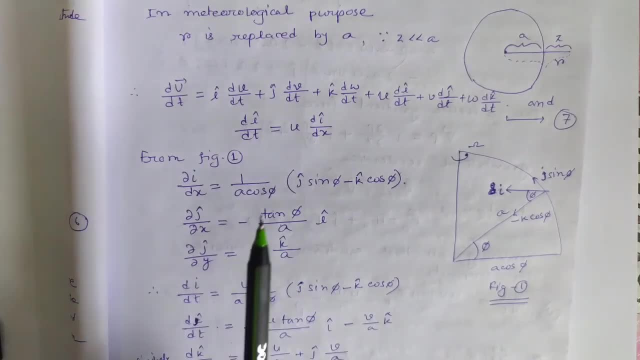 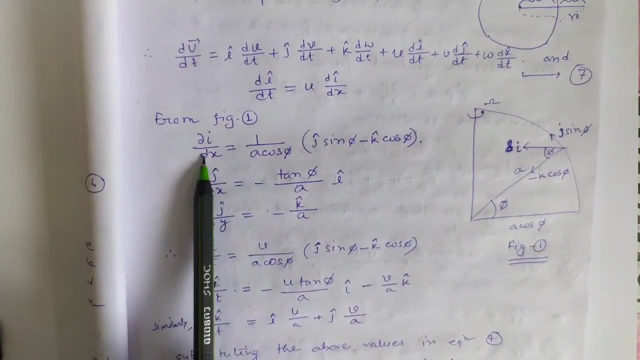 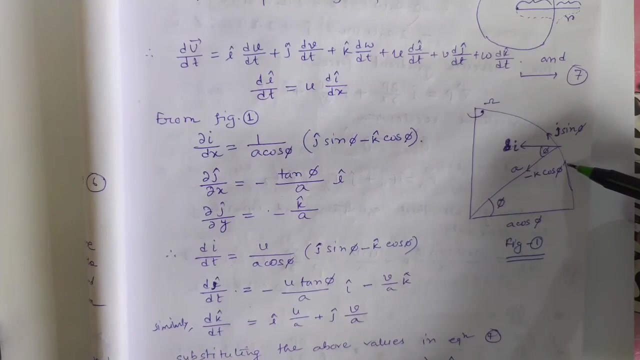 if we do not simplify also, it will we just simply we can write it. but for more clarity I am using this: di dt is equal to u di dx. from this figure you can see Now this figure shows di dx. So if we consider i, this direction, along this direction, small change in i with 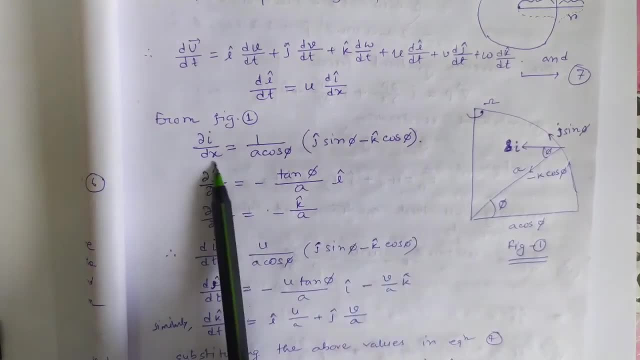 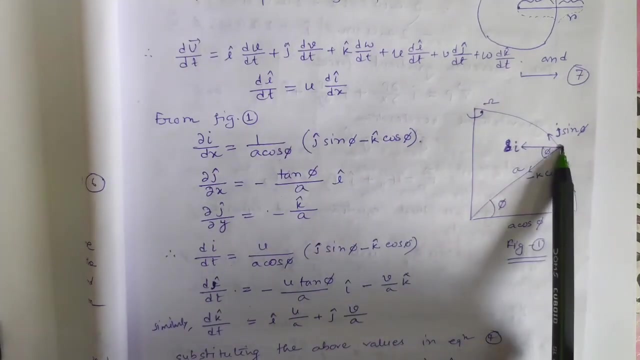 respect to x. that means this direction. we will give 1 by a cos phi So and another component. you have to consider the three dimensional picture, that is j sin phi minus k cos phi So j sin phi component will be this direction and j cos phi. 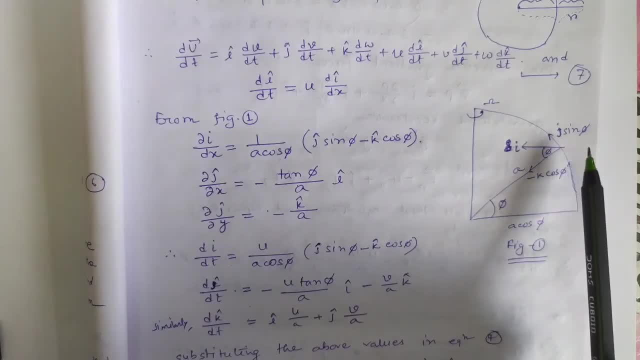 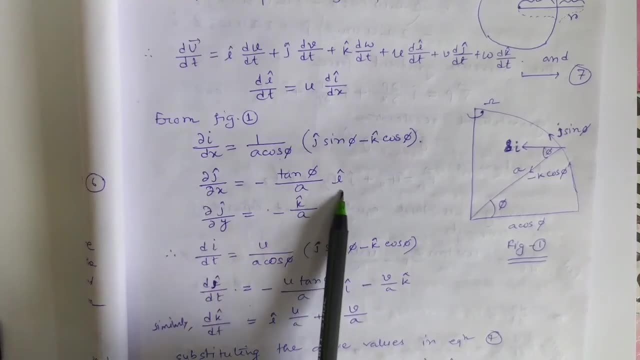 k cos phi will be in this direction, this direction, upward direction. Similarly, dj dx, dy, dj dy. we are writing and from this equation, if we put, then we are getting di dt equals to this one like u. by this one dj dt is u tan theta, tan phi. by a i cap minus v. by a k cap. 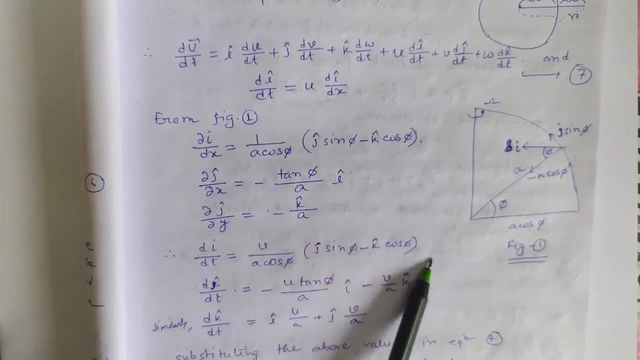 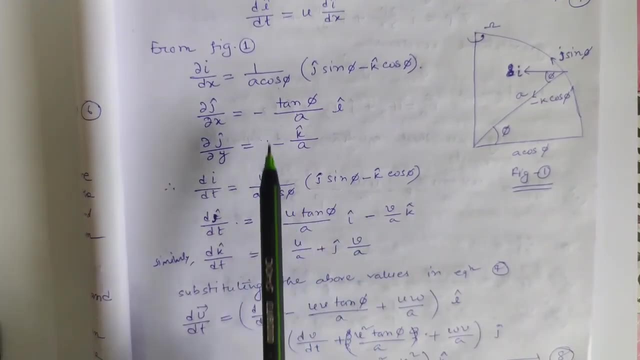 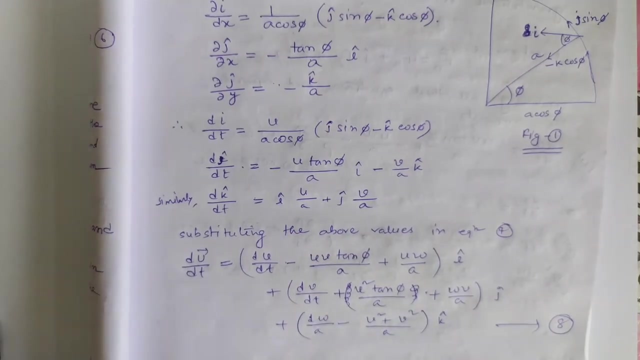 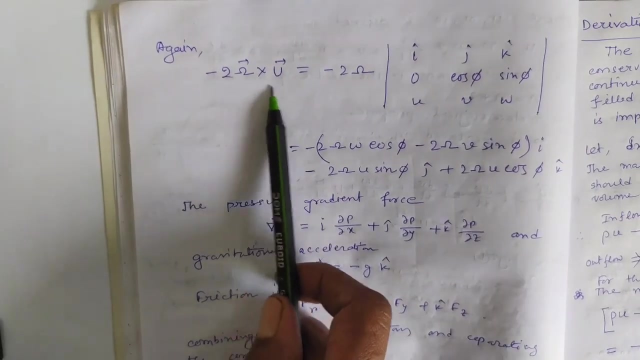 So these are the simple spherical polar coordinate transformation. Now, if we substitute these values in equation one, equation seven, we will get this one, this equation. Now the other term also we should be converted So Cross product formula if we use omega cross u, so we can write this one from there, we will. 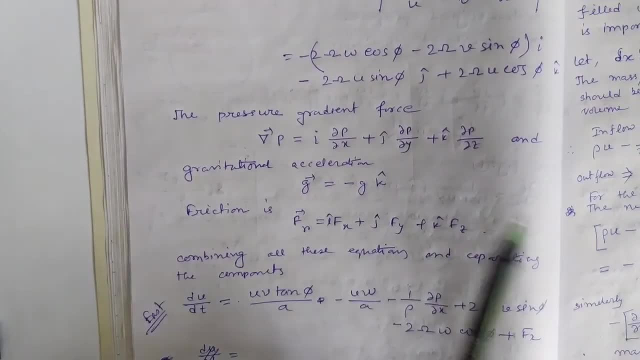 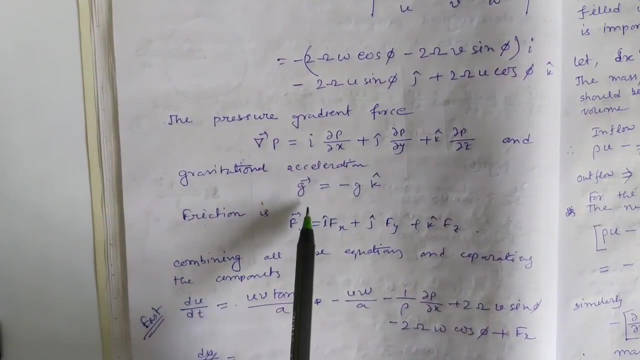 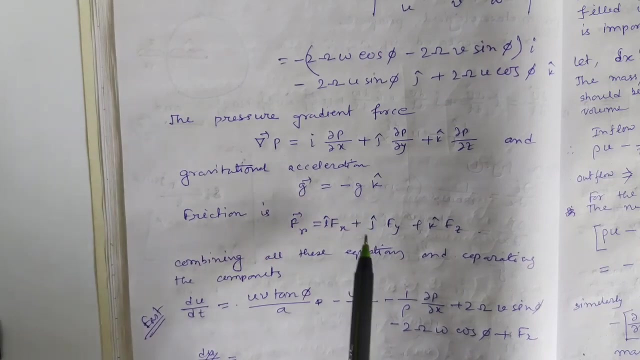 simplify the equation. and after that: another component is pressure, gradient force. we can write like this: different components: gravitational acceleration g is given by minus g, k cap. because gravitational acceleration is downward but the height is, k vector is upward. that's why negative. So gravitational acceleration only vertically. it works. that's why we use only k cap, k cap.